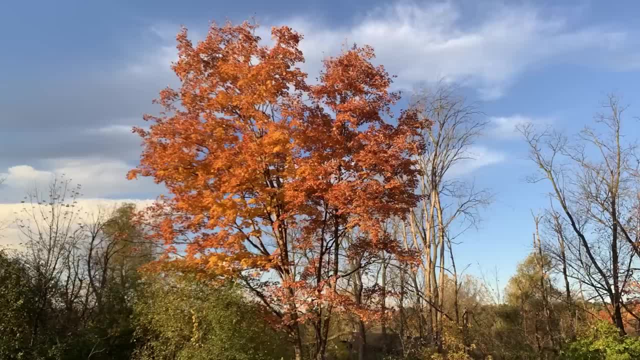 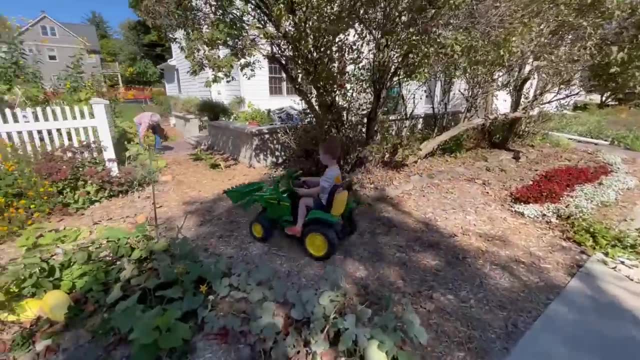 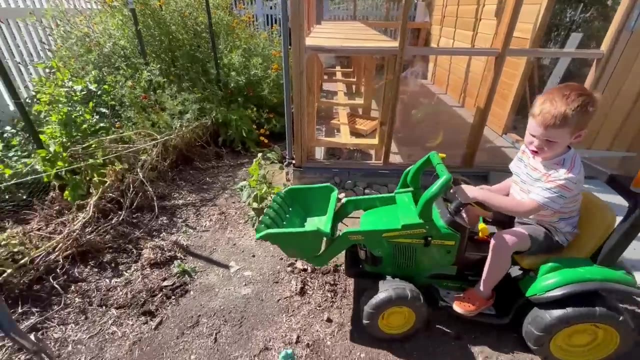 Welcome to Kid Crew. Summer is turning to fall and it's harvest time in the garden. Do you think that we can fill the scoop of our tractor with the vegetables that we dig up? Grammy's garden is full of fresh fruits and vegetables. We'll park the tractor here and start digging for potatoes. 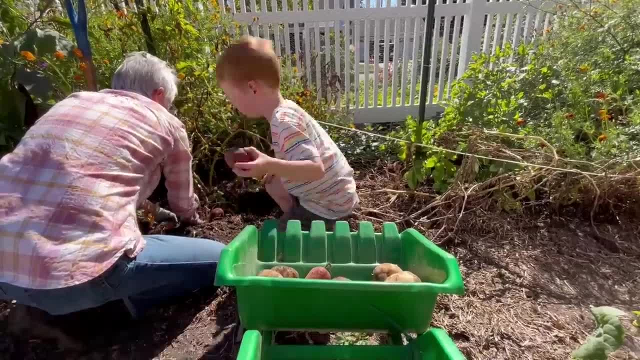 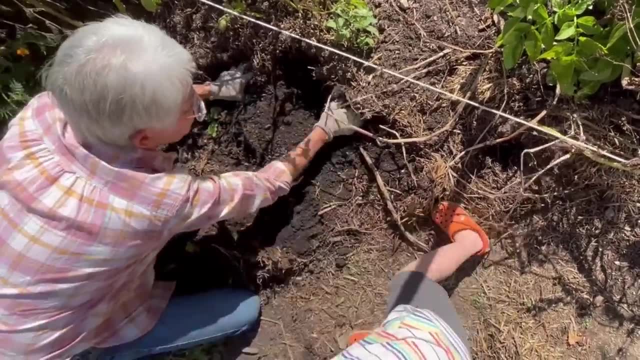 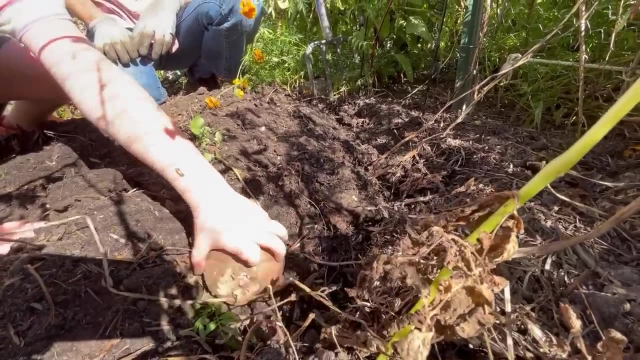 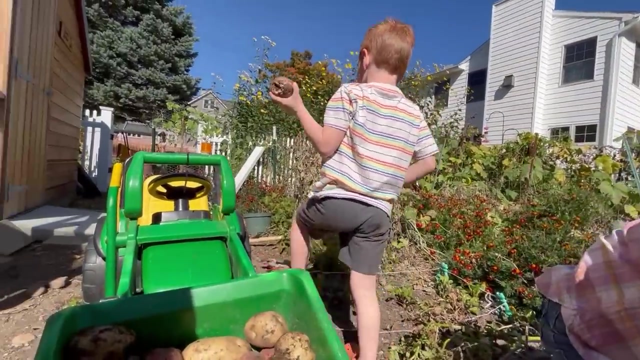 Use the shovel to loosen up the ground. Put the potatoes in the scoop. Potatoes grow underground. They'll need a good washing before we can eat them. This one has a blemish, So we won't keep that one Good throw. Now let's harvest some carrots. 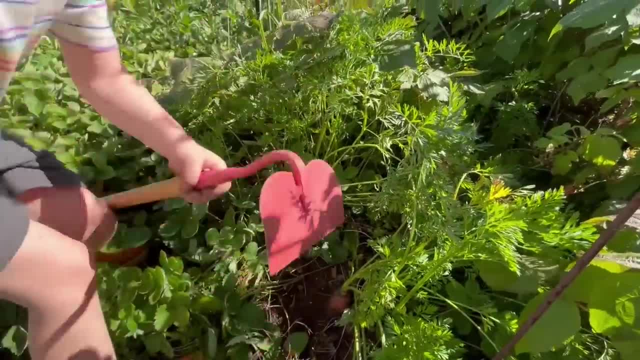 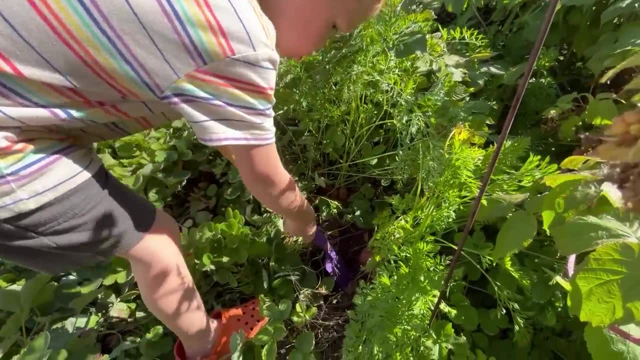 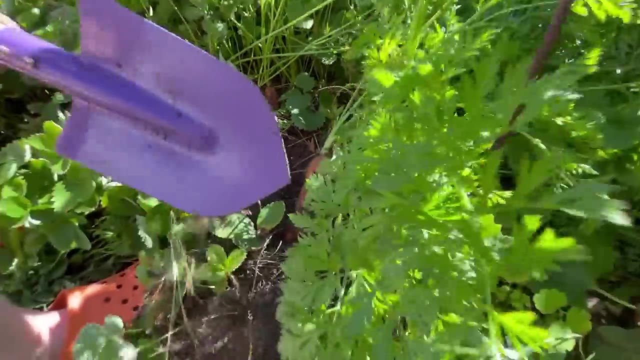 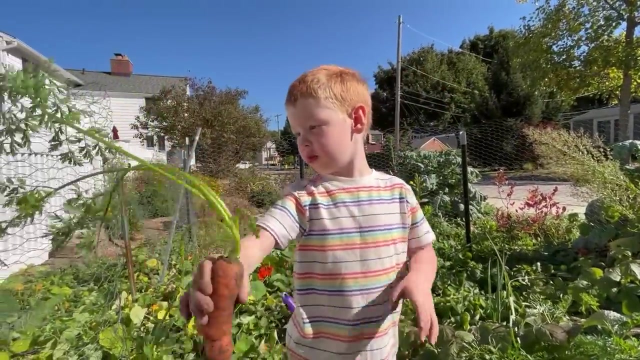 Start working the ground with a hoe, The, the, the. the shovel does a great job. Just like potatoes, carrots also grow underground, But the carrot greens that grow above the ground are also edible. Wow, Look at this ginormous carrot. It has a big stem. 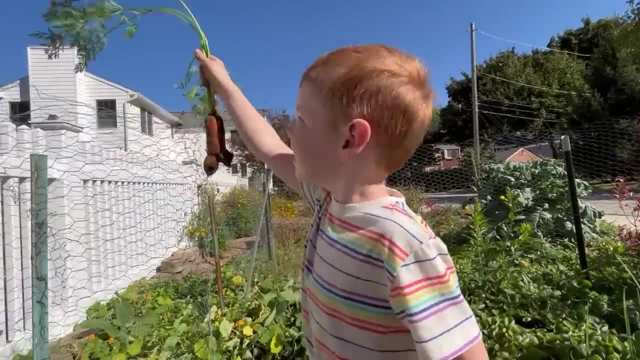 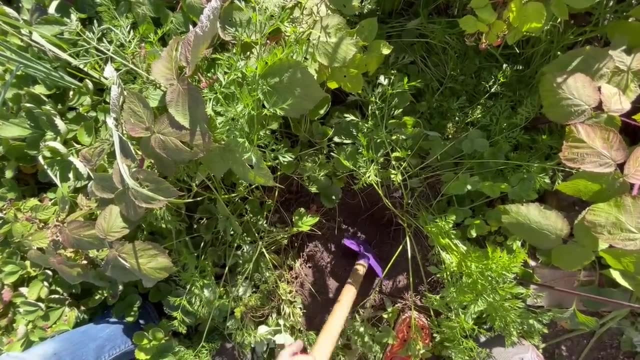 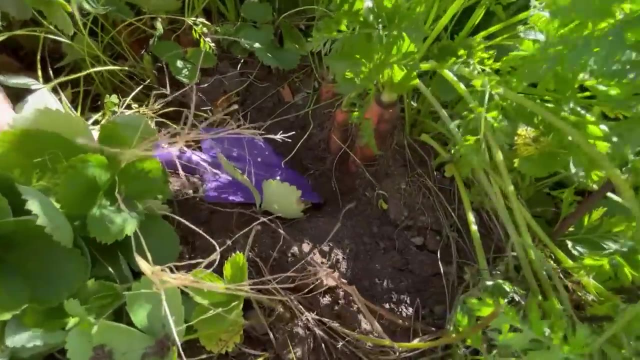 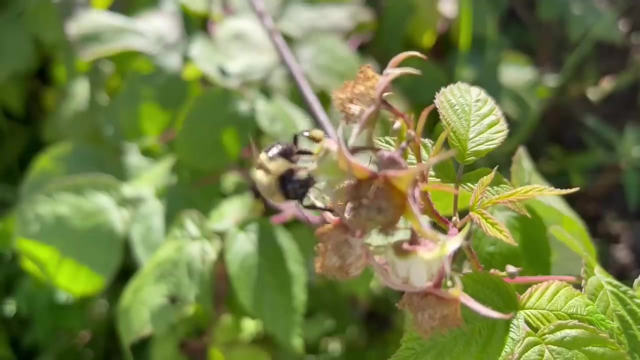 Grammy. look at that carrot. That one's just a teeny weeny, It's a. It's a family of carrots that is going to get eaten. I dig up two carrots at the same time. Bees and flowers are an important part of a successful garden. 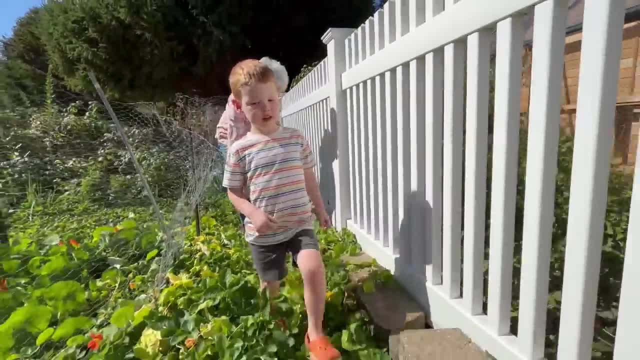 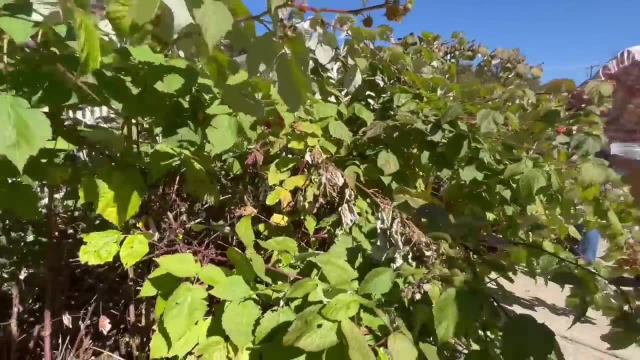 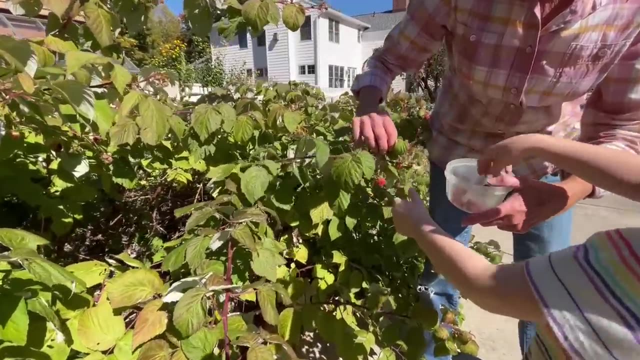 Now let's pick some juicy raspberries. A ripe raspberry is easy to pull off the plant. Here's one. I found a good one. It's a beauty. I'm going to put that one in the garden. Next up are shiitake mushrooms, which were grown on this log. 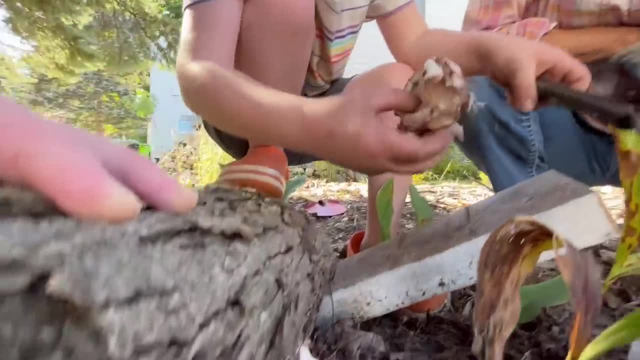 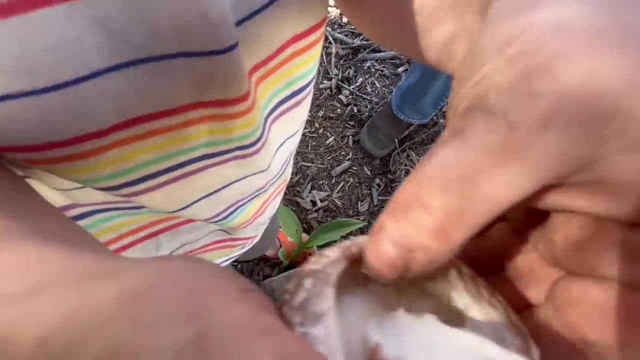 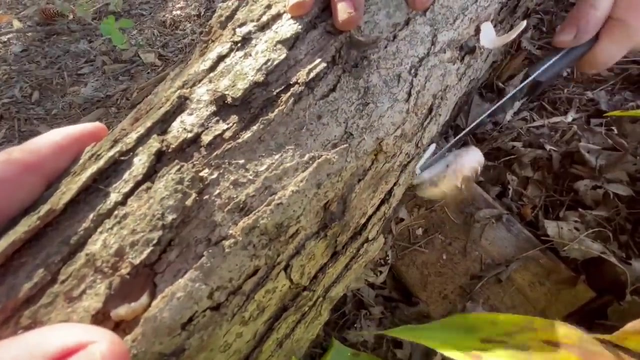 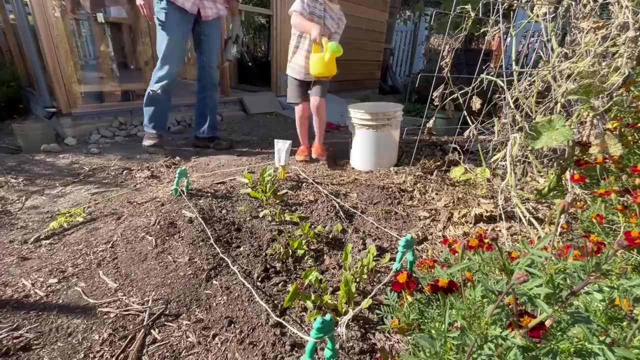 We cut them off so we have to be especially careful. It kind of feels like cheese. This part of the mushroom is called the gills. That feels like cheese. Great cutting. That's a big one. Beets were planted here and it looks like they need some water. 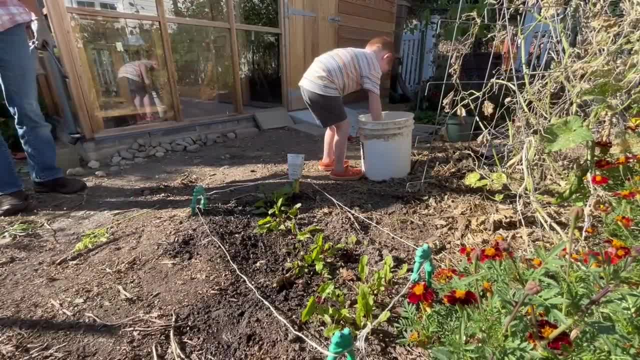 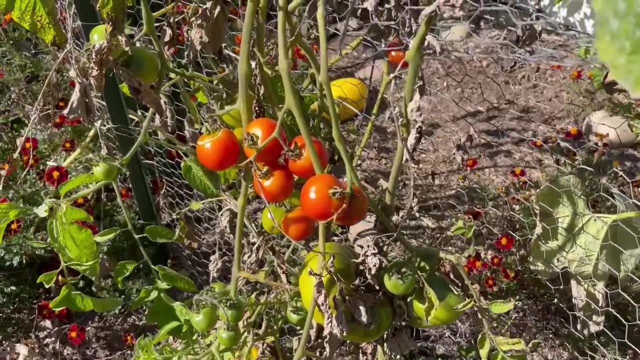 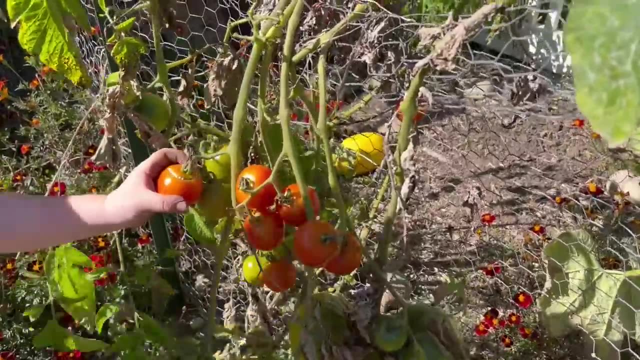 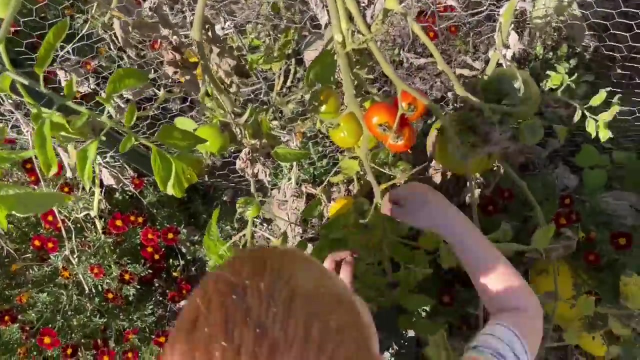 Even as the weather gets cold. these beets will be safe underground. When you pick a tomato, you just lift them up and then, if they come off, they're ready. Wow, look at all these. There are plenty of green ones that haven't ripened. 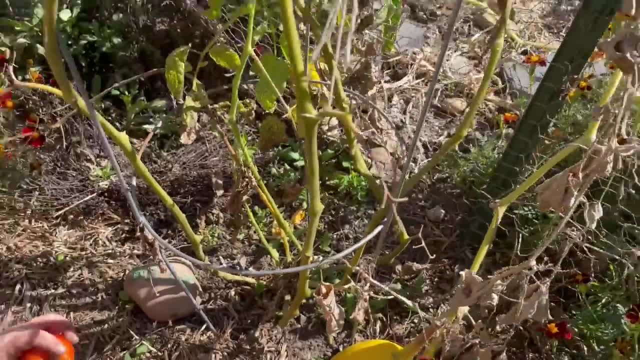 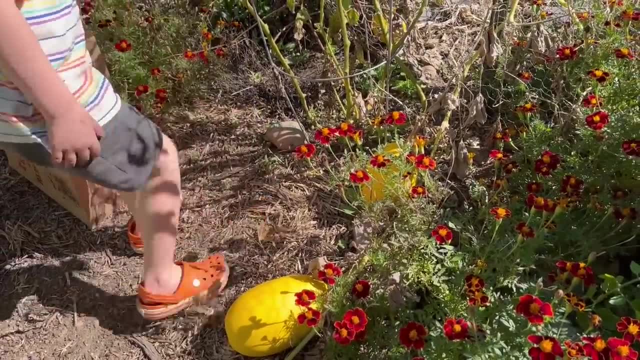 Get this one we dropped. What are those tomatoes That You want to cut? one of those? That's a hard job. I hope you can do it. Those are spaghetti squash. That looks good. That looks good. That looks good. 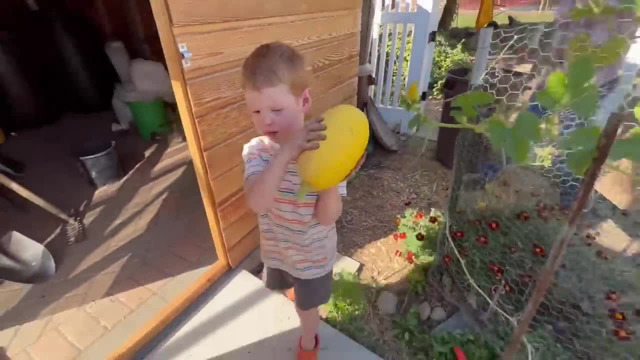 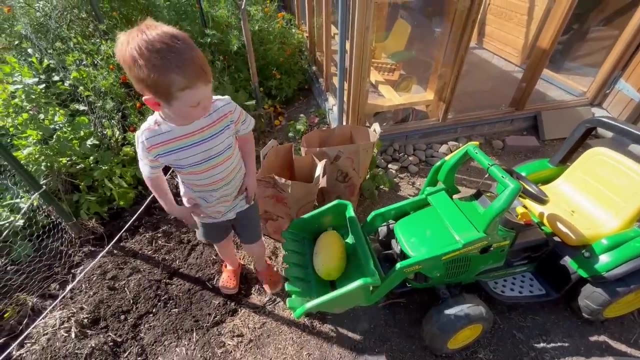 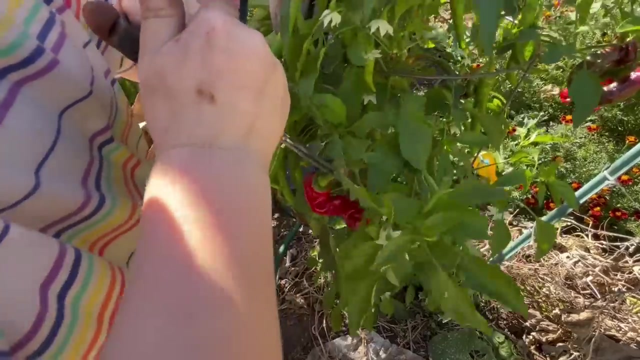 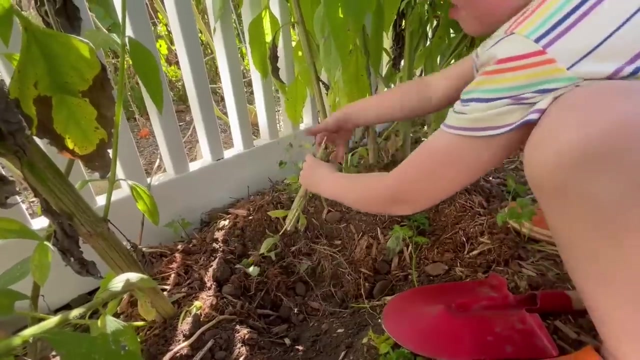 That looks heavy. That's heavy. Those are cold. Grammy has a greenhouse that will house many plants over the winter. Let's cut this pepper. I hope it isn't too spicy. This is the stem of a Jerusalem artichoke. Yank it out. 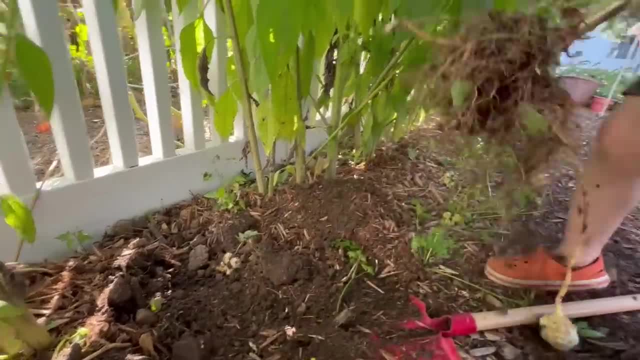 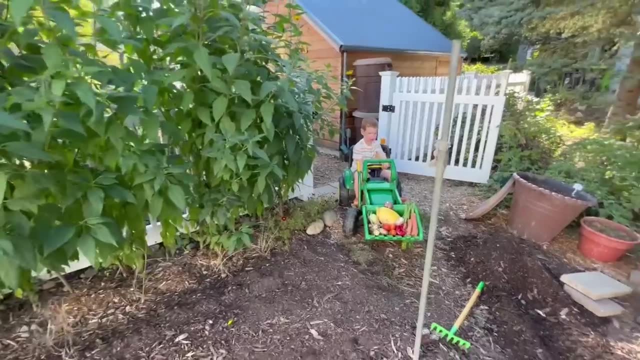 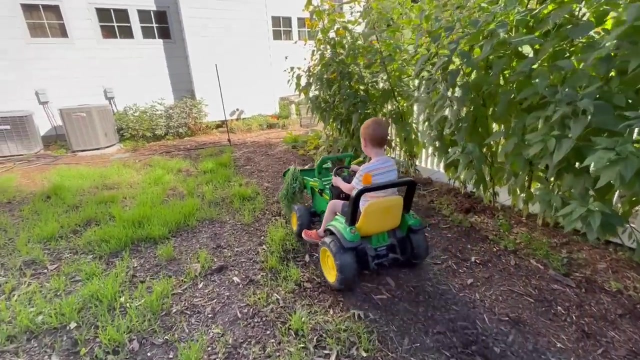 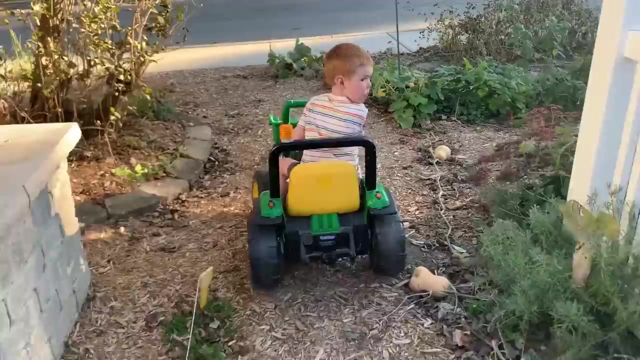 Is this one. These white things are the artichokes. We did it. The scoop is overflowing with fresh vegetables that we picked. The tractor is struggling for traction with this heavy load up front. Wow, look at how much we got Time to go home. 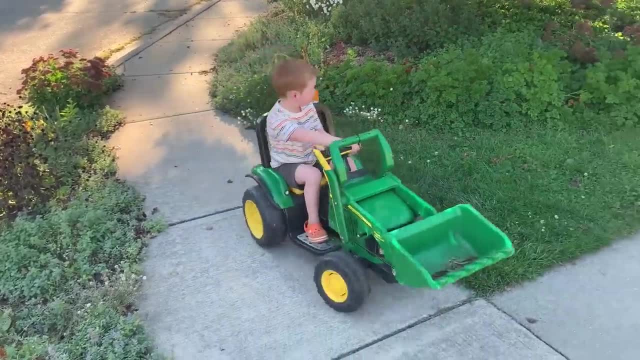 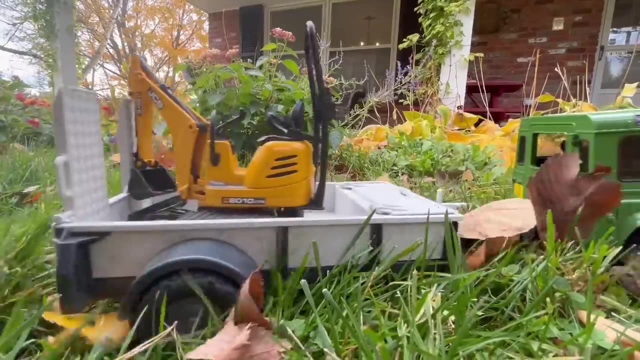 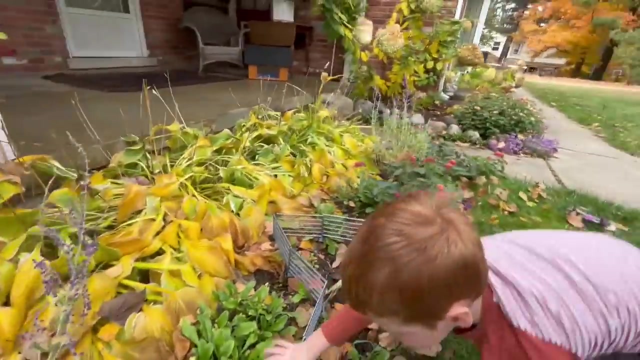 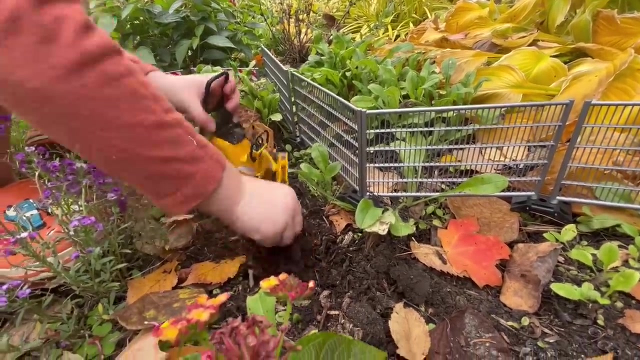 The sun is low in the sky now. Now let's plant some bulbs that will grow in the spring. We're getting help from our toys. Looks like a construction zone. It will take us days to plant the bulbs. Dig the hole with the mini excavator. 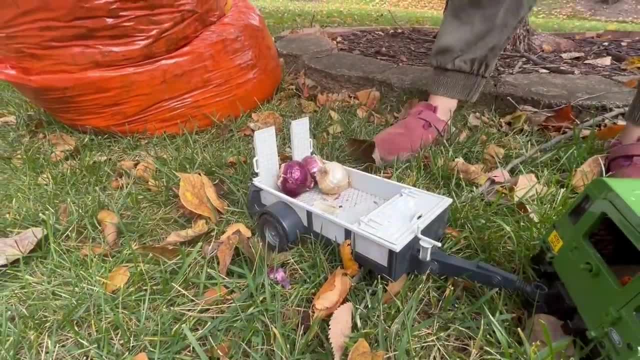 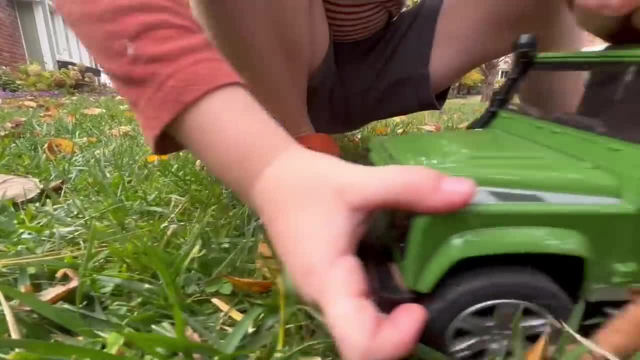 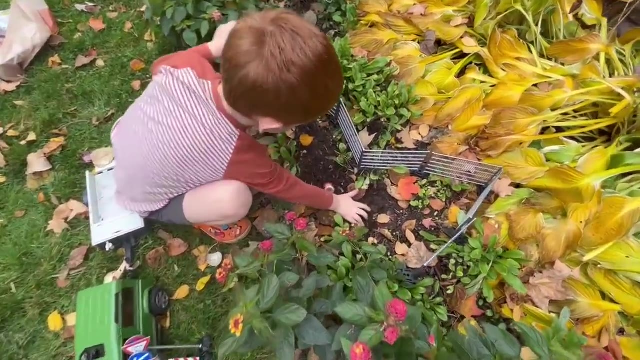 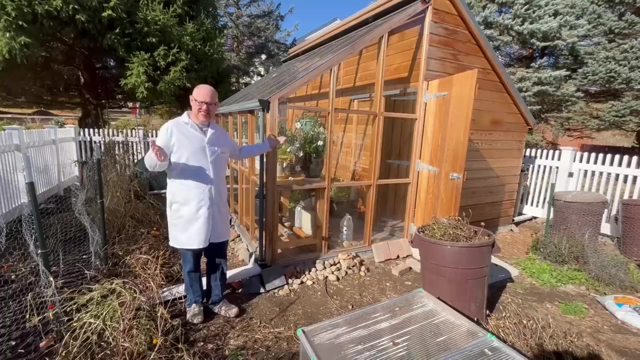 Deliver the bulbs. on the trailer They look like onions, Plop the bulb in the hole and then cover it up. Now let's learn how it works. This is how a greenhouse works. A greenhouse works by allowing the energy from the sun in while also retaining heat.